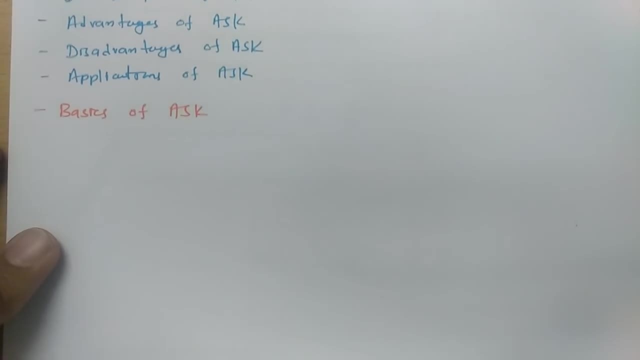 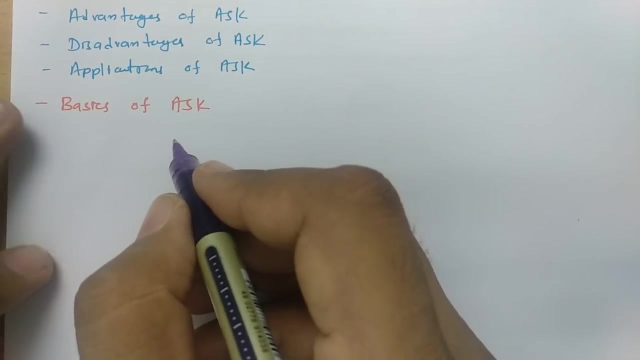 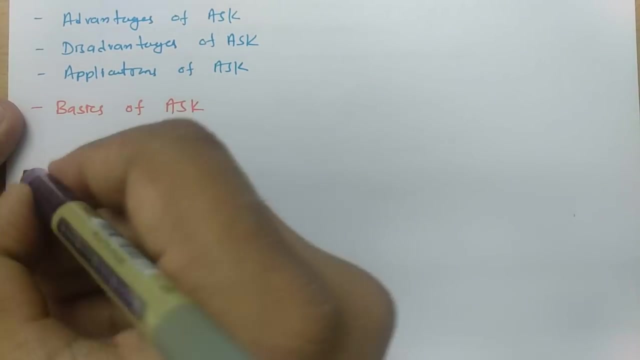 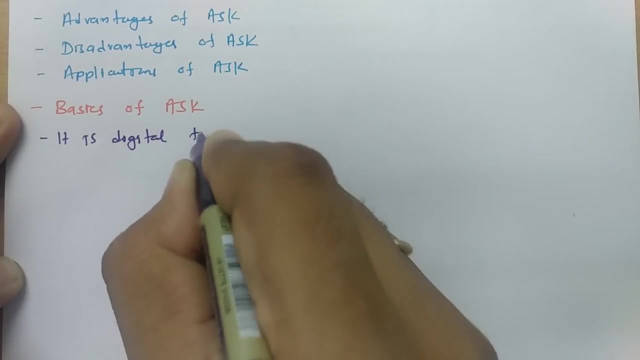 So let us begin this session with first agenda, that is, basics of ASK. Now see, when we talk about ASK- amplitude shift keying- then this is what a method which is been converting digital signal into analog signal. So it is digital to analog conversion. 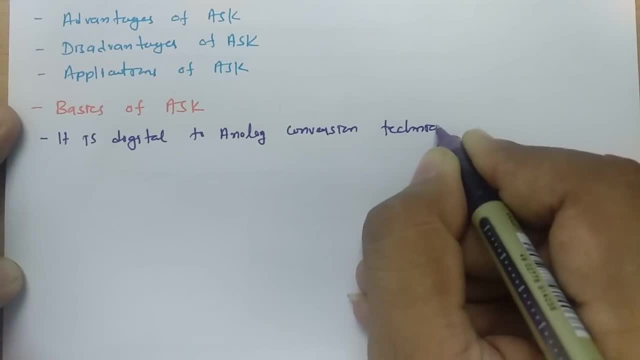 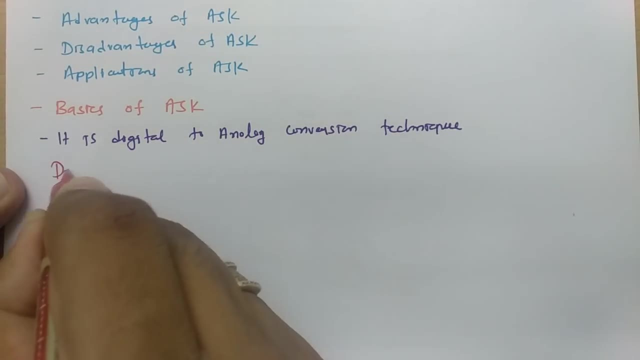 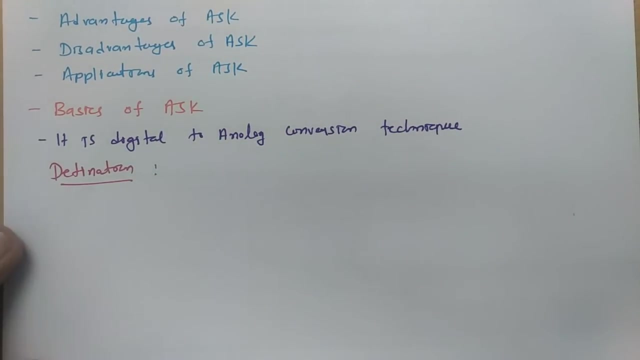 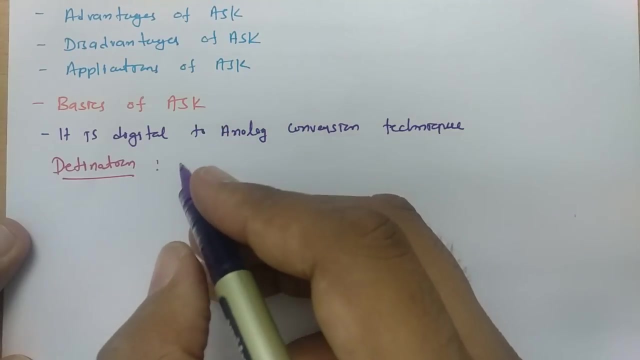 Now let us see what is the definition of it. So see, the amplitude of carrier signal varies according to the amplitude of message signal. So that is what the case, which is happening in ASK: Amplitude of carrier signal that varies with respect to amplitude of message signal. 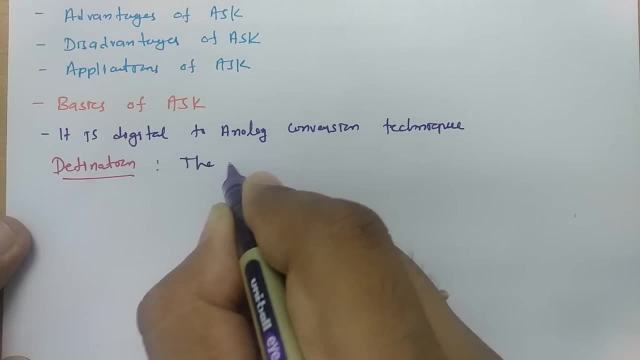 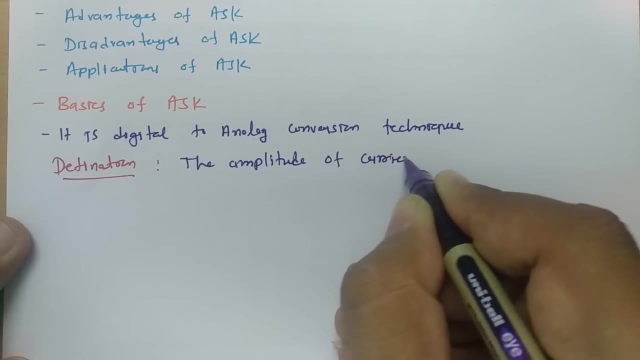 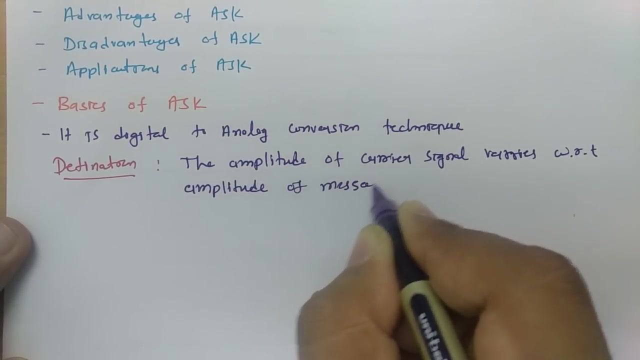 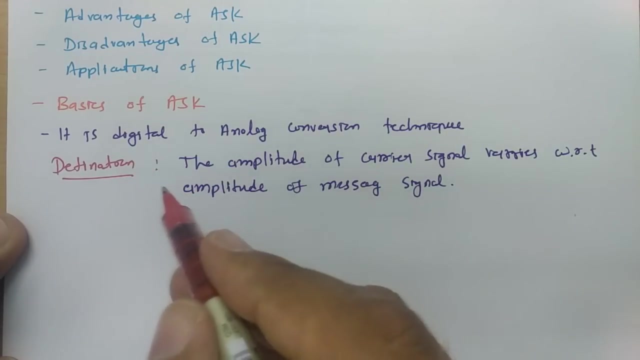 So the amplitude of carrier signal varies with respect to amplitude of message signal. Now let us try to understand how that is happening. So see here I'll consider how ASK that is been performing. So after having a waveform, one can understand how amplitude of carrier signal changes with respect to amplitude of message signal. 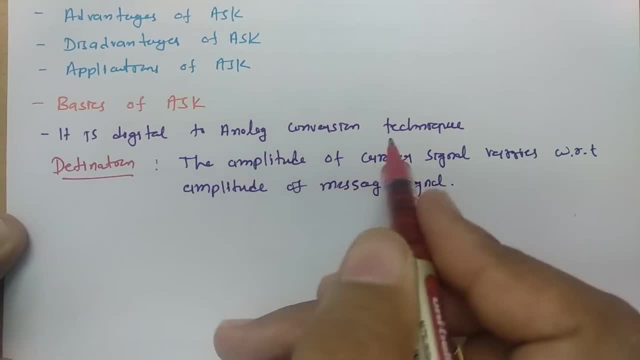 Now see, as I have told, it is digital to analog conversion technique. So we have input signal, that is digital signal. So let us say we have message signal that is empty And that is what we are giving it to multiply. And here we have carrier signal, CT, that is cos of omega CT. 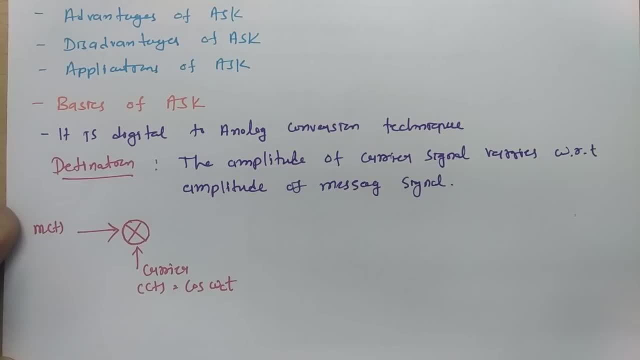 Here amplitude of carrier. that I have considered unity for simplicity, And after multiplication we'll be having amplitude shift keying output. Now see here message signal. that will be digital signal. It will be there in terms of 1s and 0s. 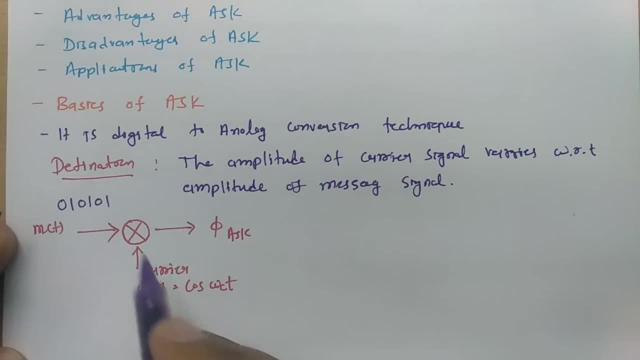 So this digital stream that will be a message signal that will get multiply with carrier signal and will be generating output. that is what amplitude shift keying. Now see how that happens. So for that, if I say I have a message signal, that is there in terms of 1s and 0s. 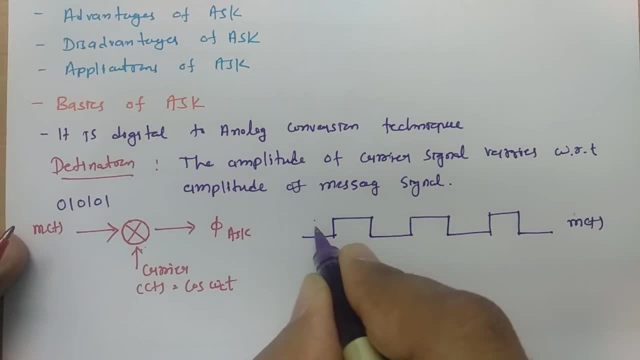 Let us say it is empty. This is 0.. This is 1.. This is 0.. This is 1.. This is 0.. This is 1. And this is 0.. So here I am, using NRZ technique to represent digital signal. 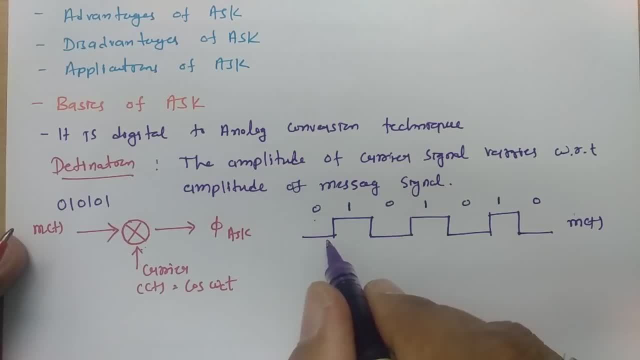 So 0 that is been assigned to 0 voltage, and 1 that is assigned to fixed voltage. It could be 1 voltage, It could be V voltage. Let us say it is high voltage. Now we have to calculate the voltage. We have a carrier signal that is high frequency carrier signal and that is having frequency omega c. 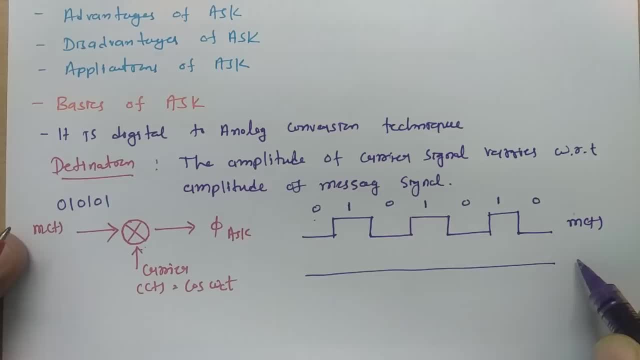 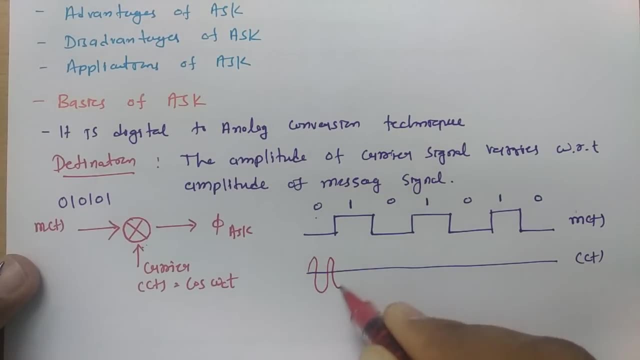 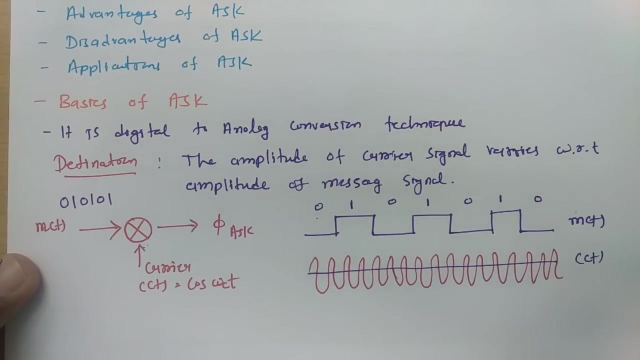 So we have a carrier signal- Let us say it is CT- And this carrier signal, that is high frequency signal. So here we are ready to generate ASK signal After having a multiplication of these two signal. So let us say this is phi of ASK. 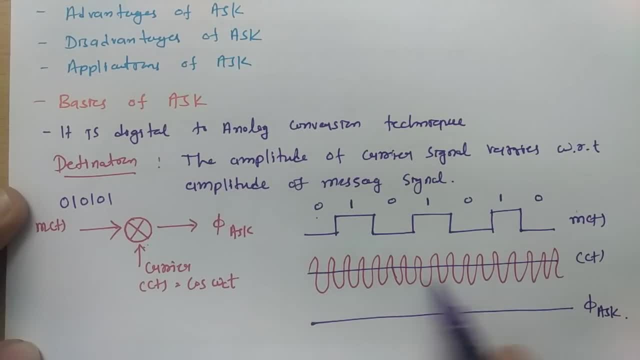 Now see what will be our output. Output will be carrier signal when 1 is there and output will be 0 when 0s are there. So if you see, for this period, there is 1.. Again, for this period, there is 1.. 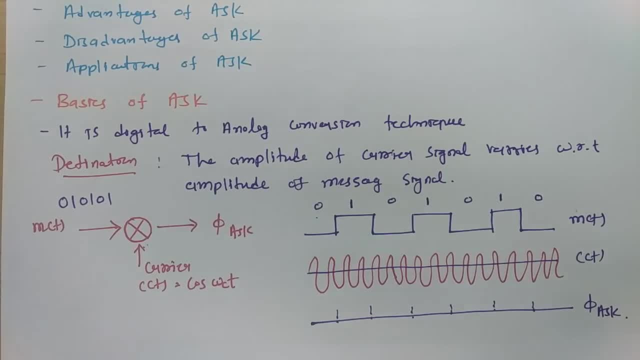 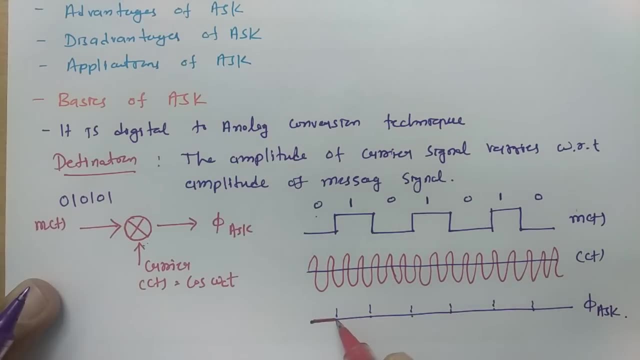 And again for this period there is 1.. So if you see your output, that will be 0 when there is 0 at message signal And when it is 1 you will be having carrier signal at output And when there is 0 there is 0 voltage. 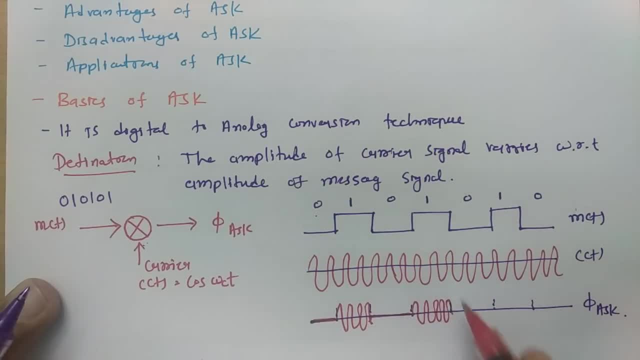 When there is 1, there is carrier. When there is 0, at that time output is 0.. Then 1 is there, at that time there is carrier. And when there is 0, at that time output is 0. So this is how our output is happening. 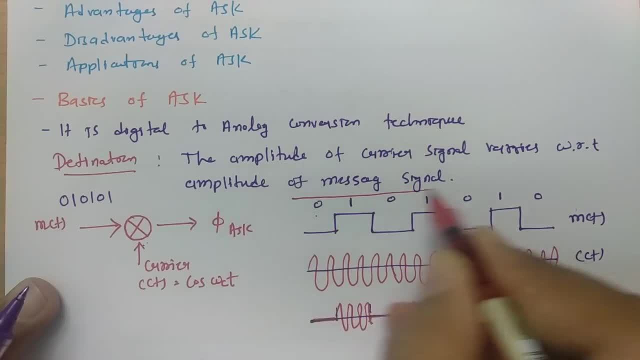 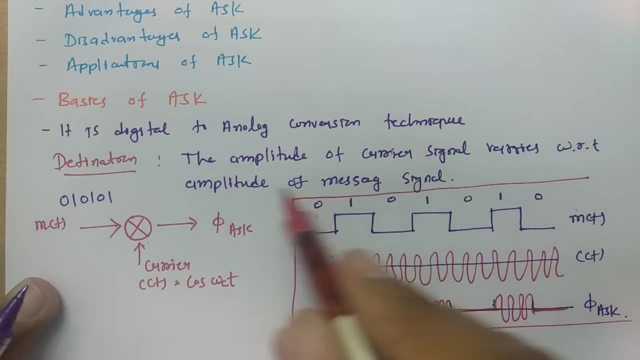 So basically, based on this waveforms, I think we can say amplitude of carrier signal varies with respect to amplitude of message signal. Now you see at output side, amplitude of carrier signal that is varying with respect to amplitude of message signal. So this is how amplitude shift keying that is performing. 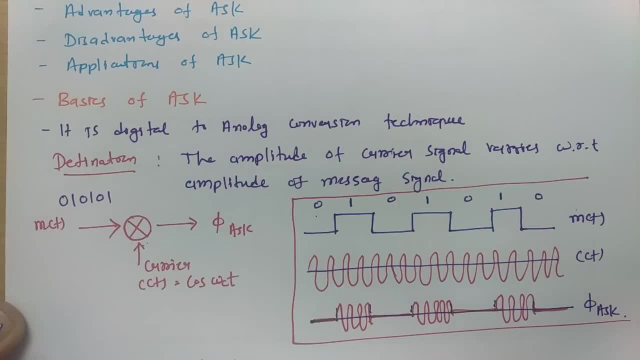 And this is how we can have a waveform. Now here, the case which we have considered, That is for binary. So for binary, For binary n is equals to 1.. And when n is equals to 1. This ASK that is even referred as 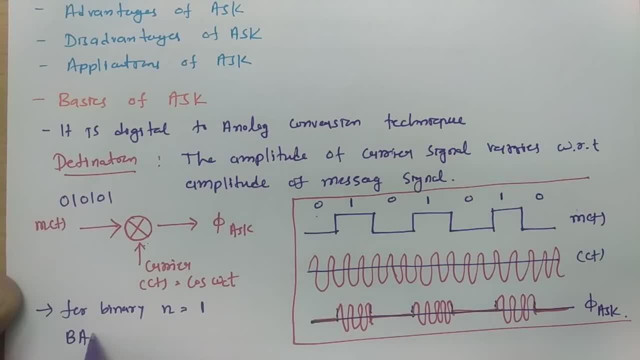 Binary ASK And even you can say it is ON OFF Shift keying. It is even referred as ON OFF keying. So For binary n is equals to 1. And that is even referred as Binary ASK or ON OFF keying. 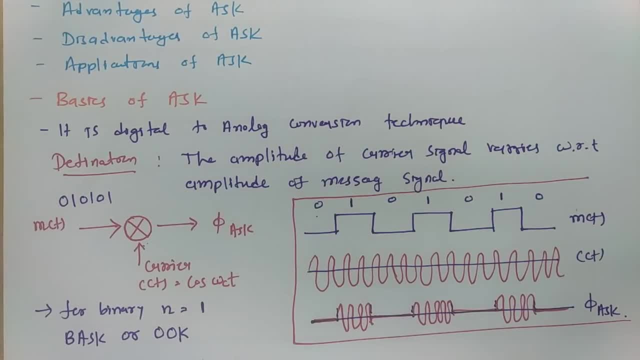 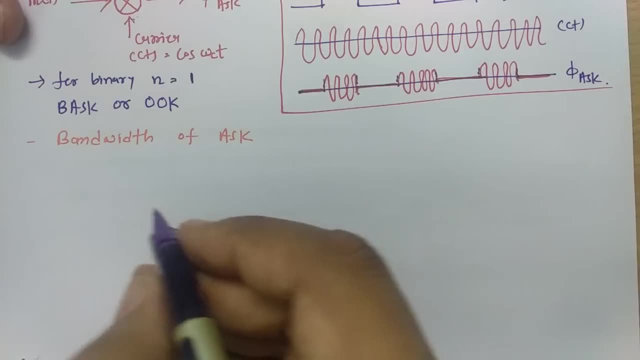 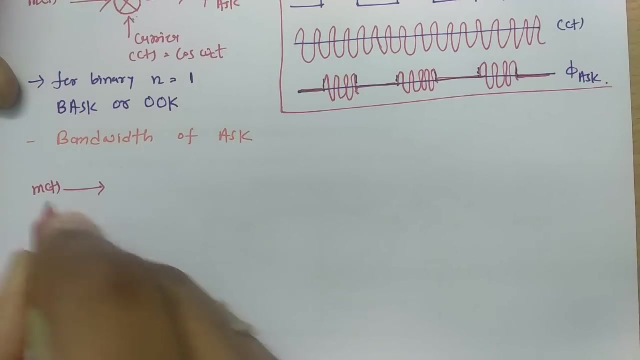 So I hope that this basics, that is clear to all. Now let us move on to next part, That is, Bandwidth of ASK. Now see As I have explained That ASK: All we need to do is We need to multiply. 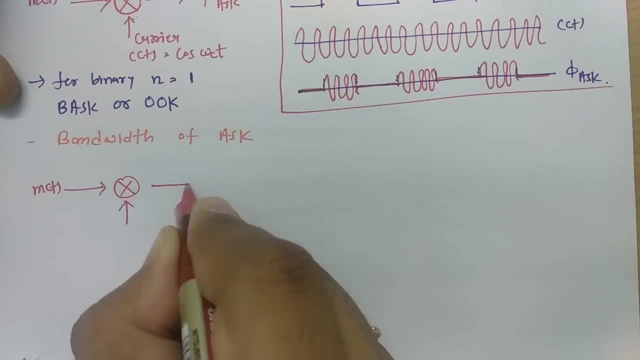 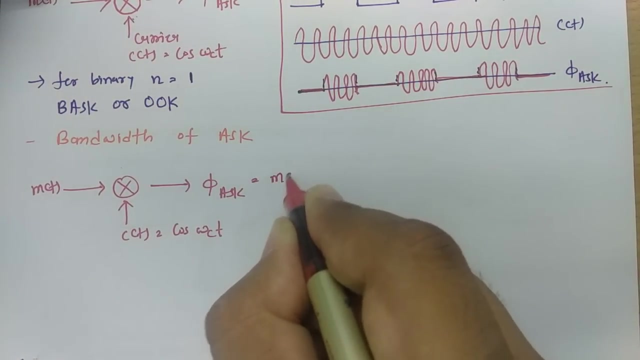 Digital message signal With carrier signal And you will be generating ASK output. Now, here you will be finding This ASK output That is composite signal Of this message signal And carrier signal. Practically, it is multiplication Of this two signal. 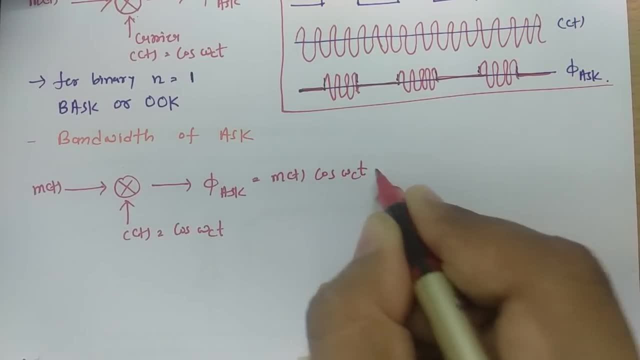 So that is mt into Cos of omega Ct. So bandwidth Of this ASK That is directly proportional to Baud rate of Message signal. So if I say I have a bandwidth, So that is what directly proportional to. 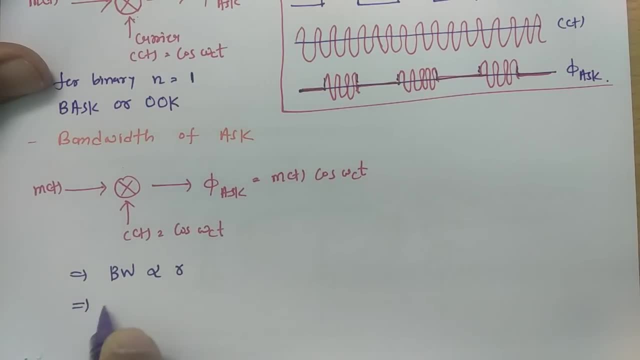 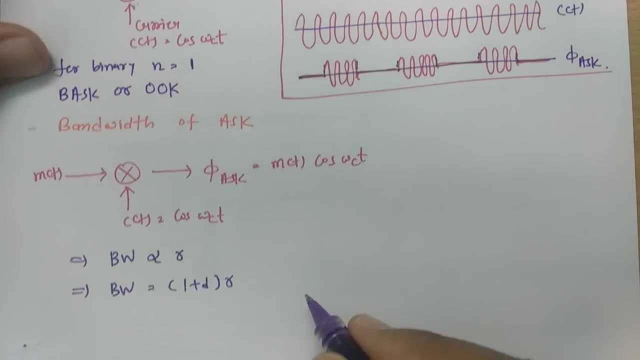 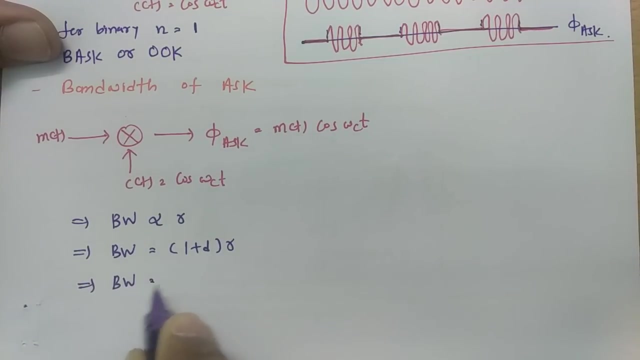 Baud rate So that proportionality constant, That proportionality constant, That is 1 plus d Into r. Now you can see in my previous session Where I have explained Baud rate, that is data rate by n. So bandwidth is equals to. 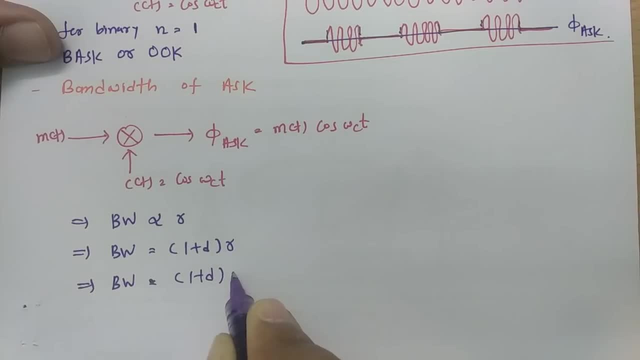 1 plus d Into Capital r by n, Where capital r is data rate And n is Number of bits required to represent 1. Sample. So let us try to understand How many parameters that is there In this bandwidth formula. 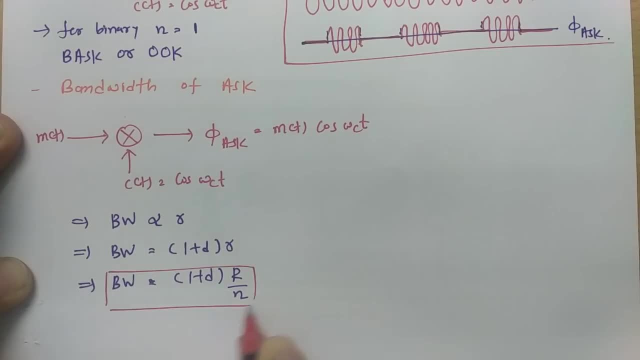 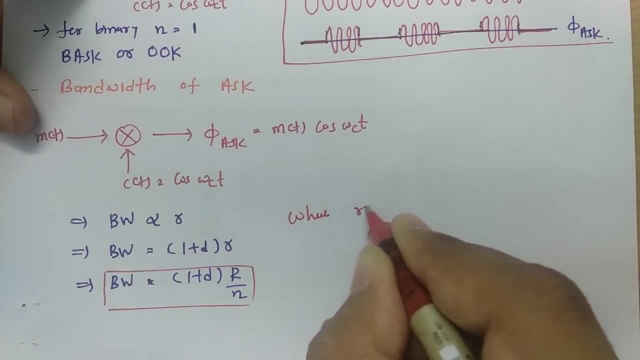 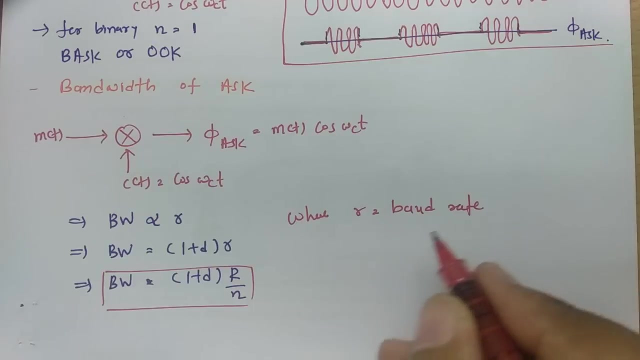 So it will be more clear How we can utilize this formula In solution of examples. So here We can say here: r, that is Baud rate. Now I have already Explained what is baud rate. You can see my previous session. 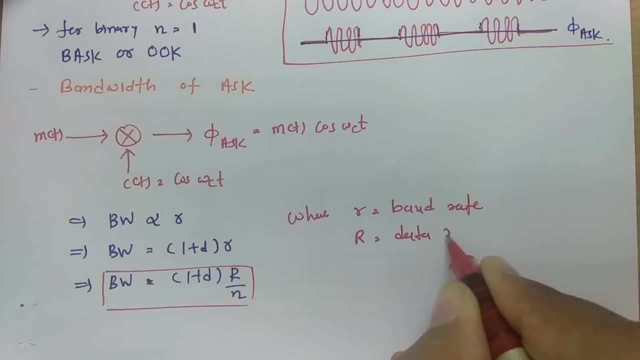 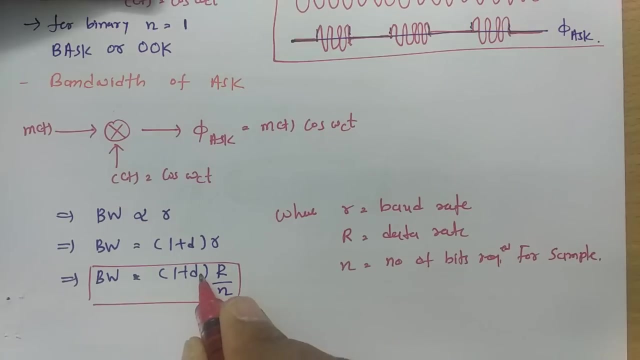 Capital r, that is Data rate, Small n, That is Number of bits Required For Sample, Or one can say For Elements. And here New parameters, Small d that is appearing. So what is this small d? 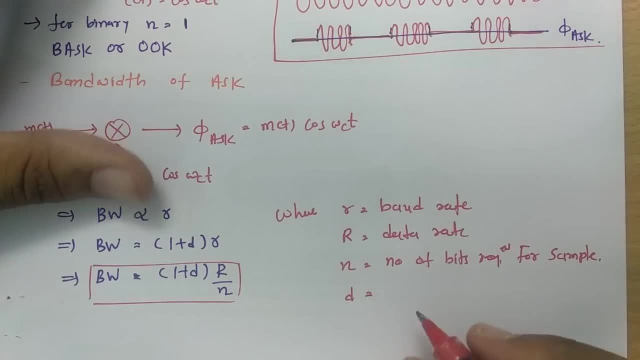 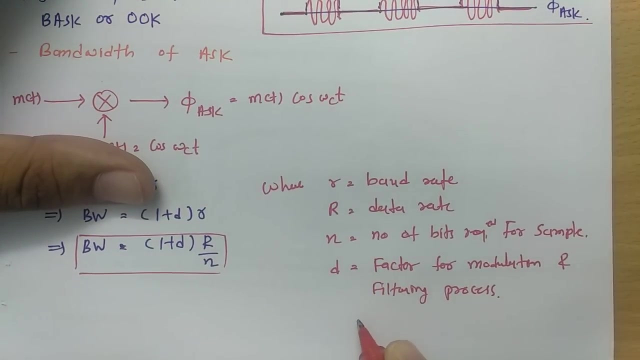 It is a factor For modulation and filtering process. So d is A factor For Modulation And Filtering Process. Now see Range of d. Range of d That is There in between 0 to 1.. 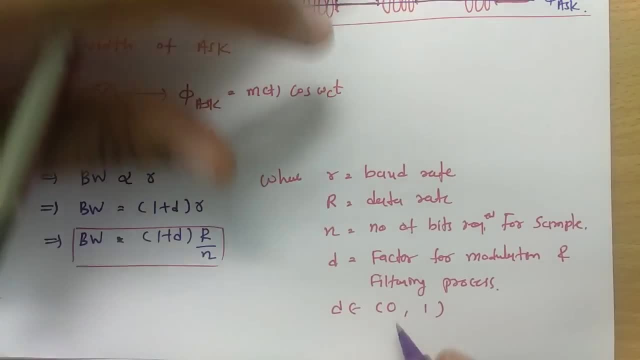 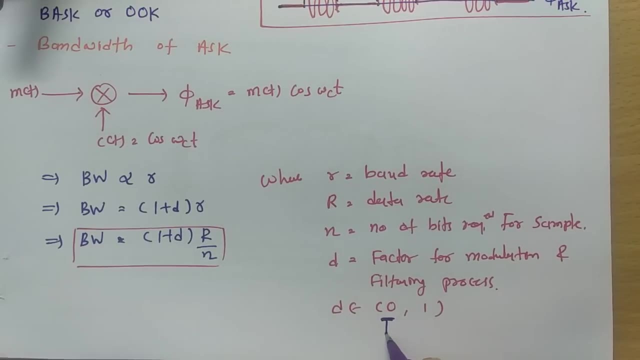 Range of d There in 0 to 1.. For ideal modulation: For ideal modulation, d is equals to 0. So d is equals to 0.. For Ideal Modulation, And d is equals to 1.. 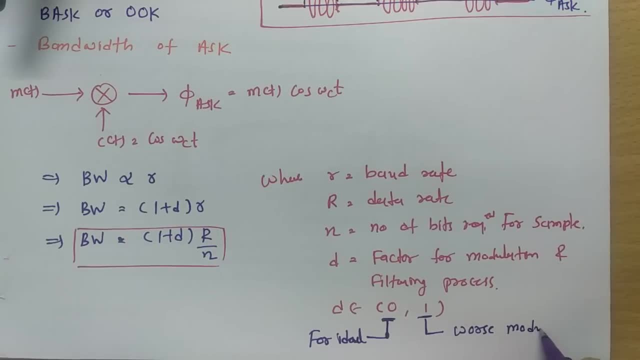 For Worst Modulation, D is equals to 0. for ideal modulation And d is equals to 1. worse case. so if you want to calculate bandwidth for ideal case, you will be finding bandwidth is equals to. if you place D is equals to 0, bandwidth is: 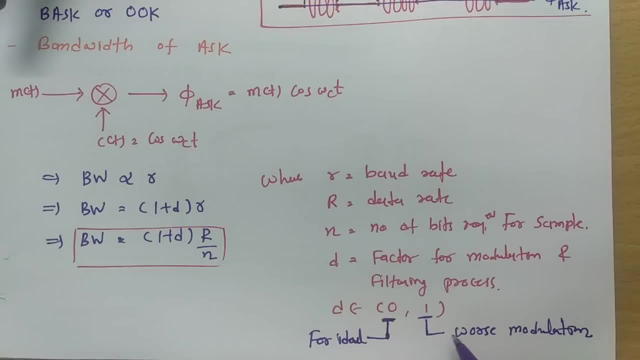 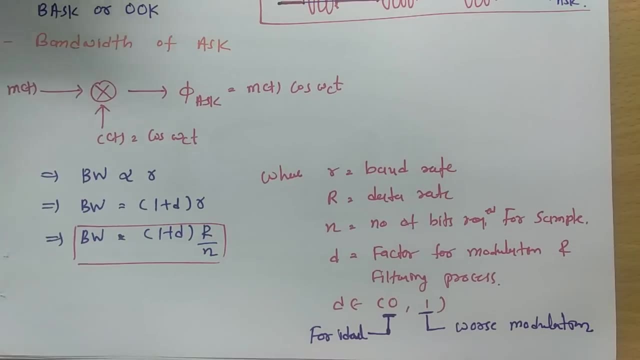 equals to R. and for worse modulation, if you place D is equals to 1, you will be finding bandwidth is equals to 2, R. so for ideal case, for ideal case, you can say bandwidth that is equals to R and for worse case, you can say bandwidth. 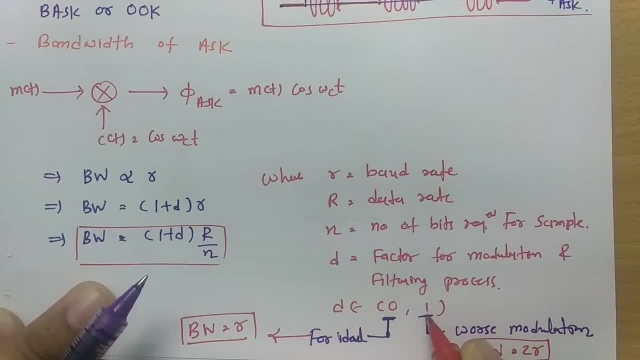 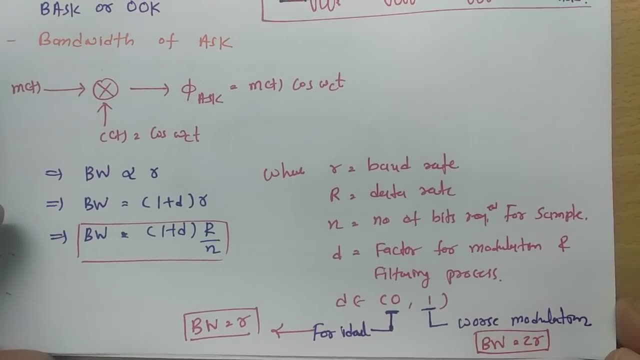 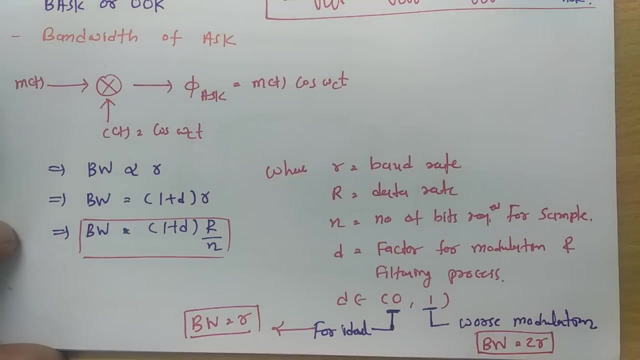 that is equals to 2 R. the reason is: D is equals to 1. if you place D is equals to 1 in this, you will be finding worse modulation and in that case bandwidth will be 2- R. so see, this is how we can have a calculation of bandwidth now see. 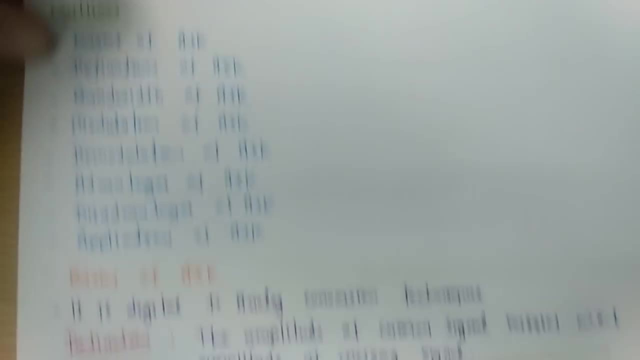 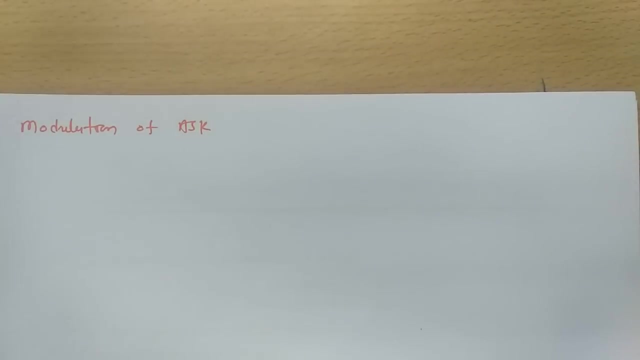 I'll explain modulation and demodulation of ASK. so that is very helpful to understand how exactly ASK is functioning. now see what is modulation. modulation is a process of generation of ASK. so I have already explained earlier: by multiplying digital signal with carrier signal we can have ASK. so you can see, here we have carrier. 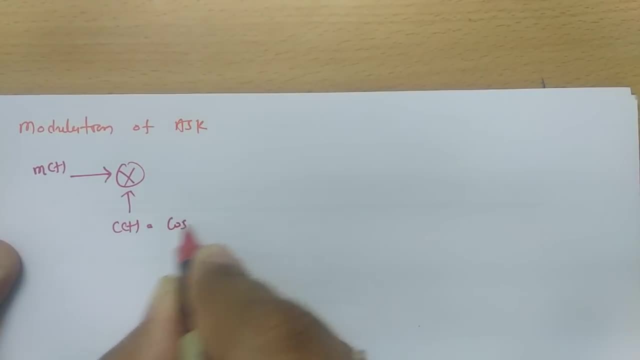 signal and this is message signal. if I say carrier signal is Omega C T, message signal is M T, then after multiplication ASK signal that will be M T into cos of Omega CT. so by multiplying message signal and carrier signal we can have a modulation of ASK. 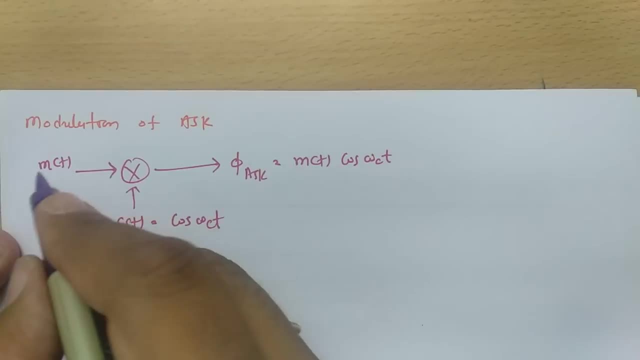 and here we can say: empty. that is there in terms of digital signal: 1, 0, 1, 0, like this. So we can say this mt, that is 1 or 0,. 1 is there for positive voltage and 0 is there for no voltage. 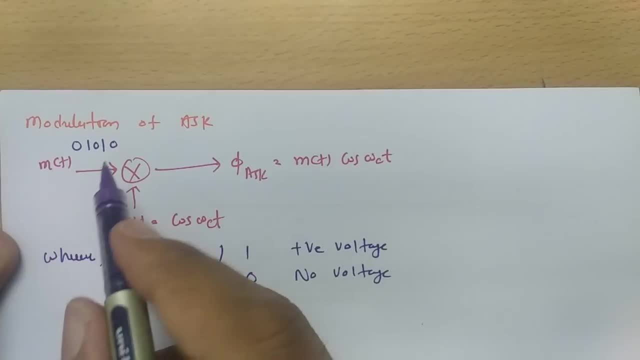 So this is how mt is there. The reason is mt is digital, so it will be there in terms of 1s and 0s. So 1 is there for positive voltage and 0 is there for no voltage, And that is how we can have a modulation of signal for ASK. 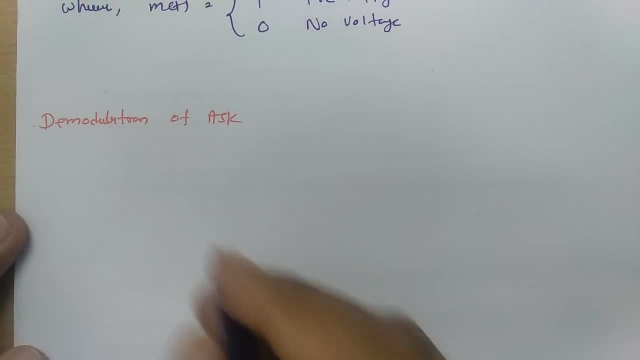 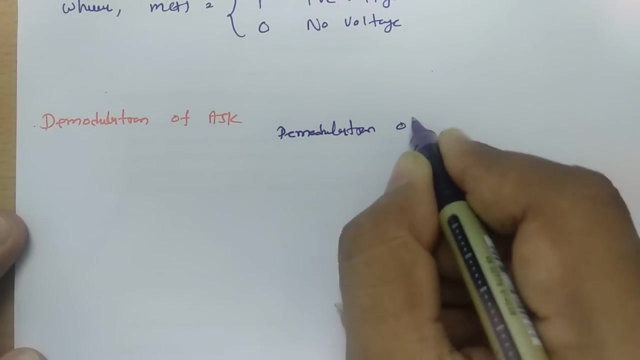 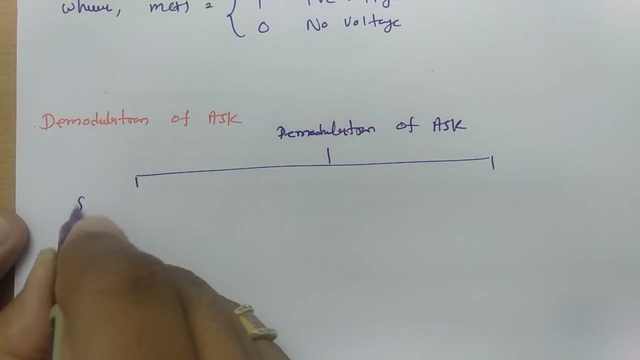 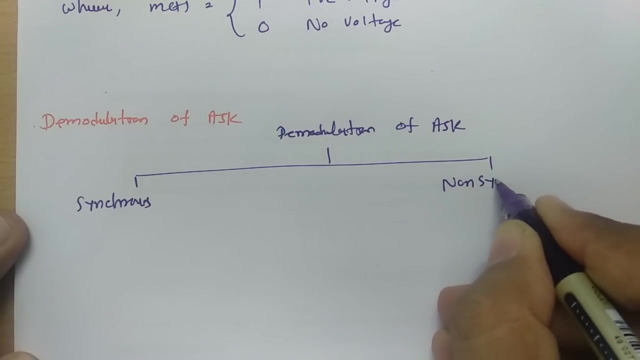 Now let us talk about demodulation. So when we talk about demodulation of ASK, then there are basically two methods which we can have. One is synchronous method And second is non, And third is non-synchronous method. 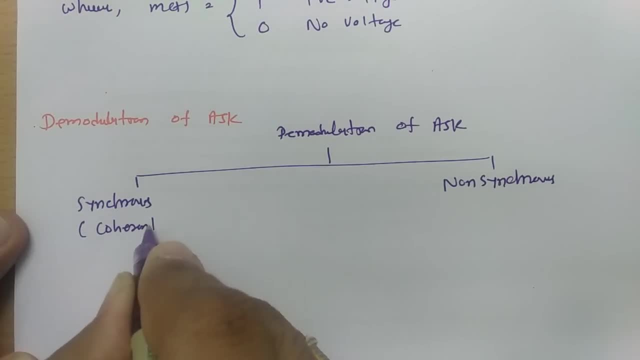 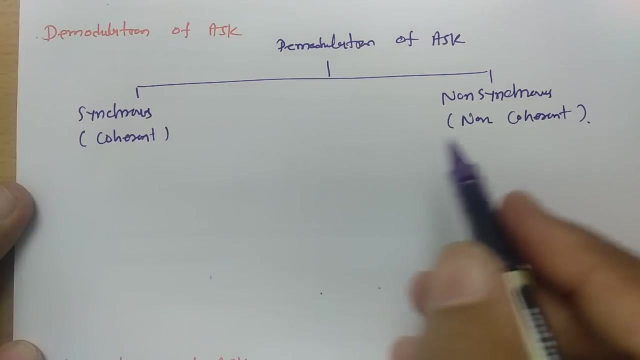 Synchronous means coherent. Non-synchronous means non-coherent. Now see, both of these methods are having some advantages and some significance. We will discuss comparison with advantages and disadvantages of both. So let us try to understand this. Now see, 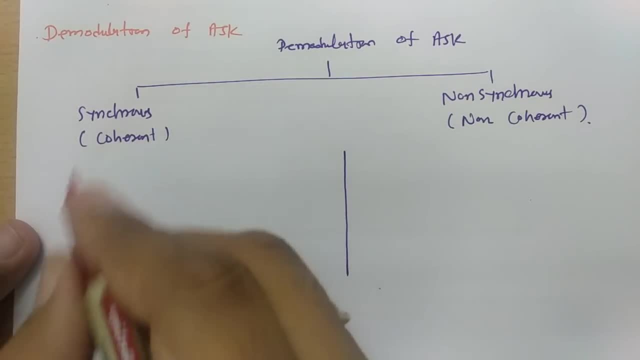 When we talk about synchronous, coherent detection. So in that case all we do is we have modulated signal which we receive. So the signal which we are receiving that will be mt, cos omega ct. that is what ASK signal. Now when you multiply this signal with carrier signal- cos omega ct- you will be finding, after multiplication: 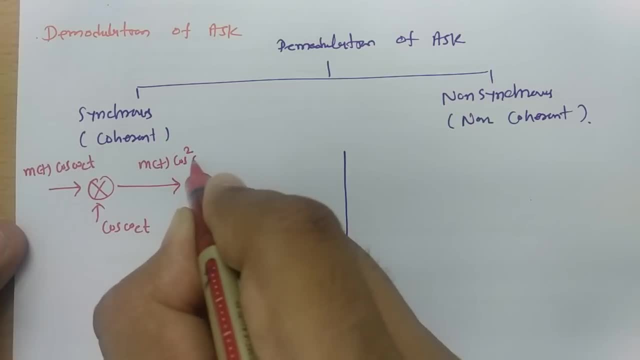 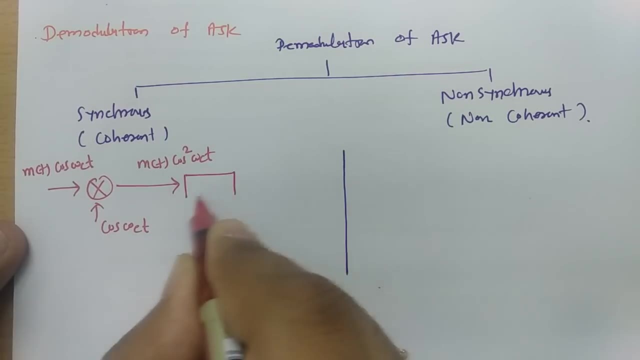 this signal will be mt cos square omega ct and when you pass this mt cos square omega ct signal through low-pass filter, you will be able to receive original message signal. So see, this is how we can have synchronous or coherent detection. So in coherent detection we need to have oscillator. 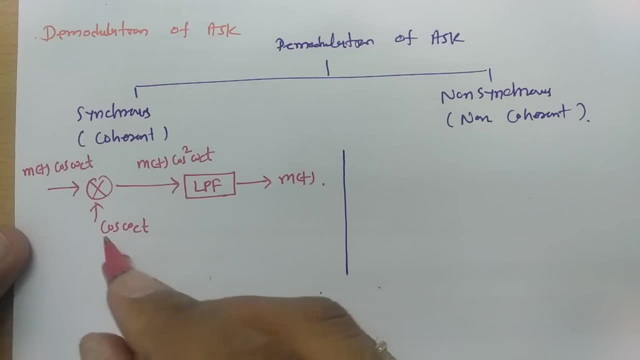 In coherent detection we need to have oscillator. So in coherent detection we need to have oscillator. And this method is efficient, but its cost is high. And this method is efficient, but its cost is high. Why The reason is we need to have oscillator here as a carrier. 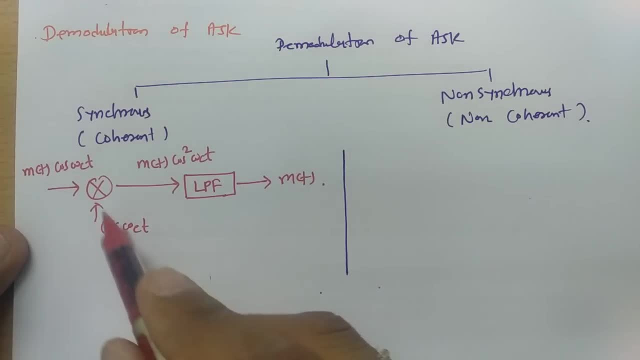 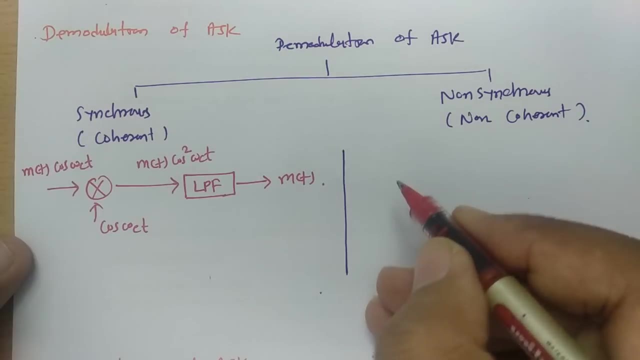 to multiply it with received signal. So this method is efficient, but it is costly. Now see when we talk about non synchronized coherent detection. so I did time. all we do is we pass this modulated ASK signal through this. 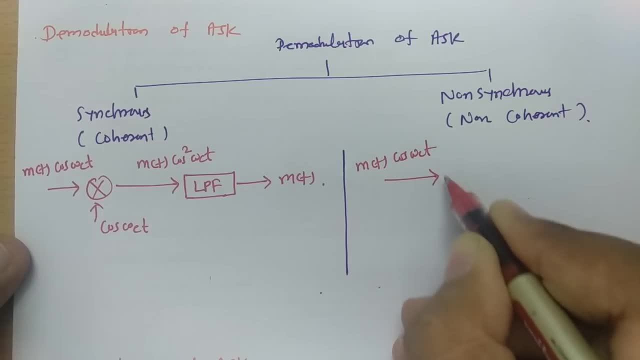 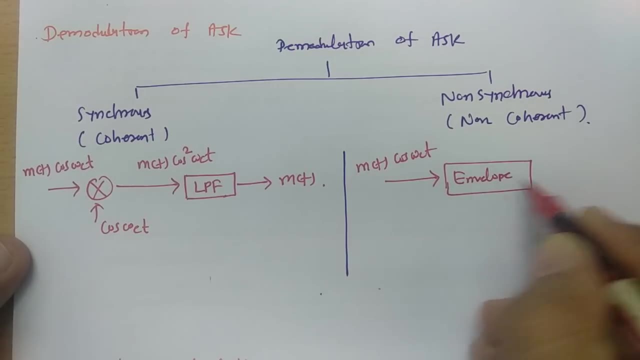 that is, mt, cos, omega, ct, through envelope detector, and when you pass it through envelope detector you will be able to receive message signal. So here, in this method, we don't need to have any carrier signal. Now see, I am not going to explain you how envelope detector functions. 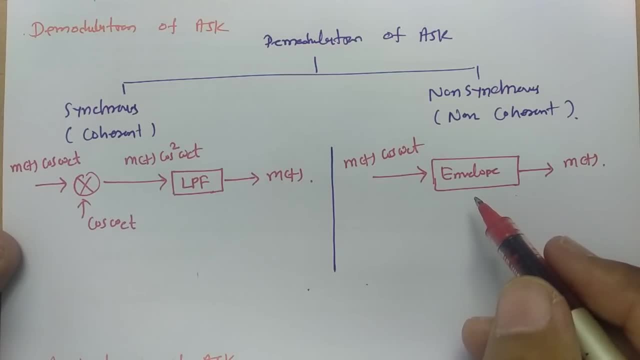 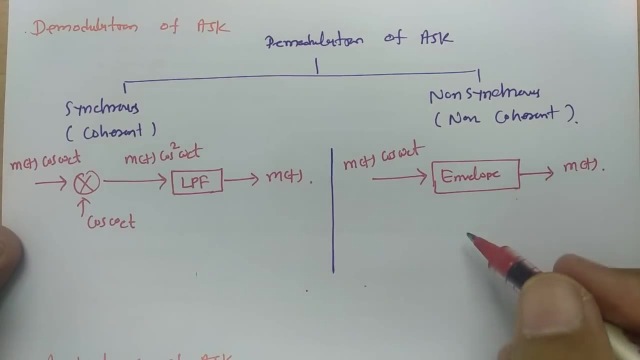 you can see my analog communication playlist where I have explained different methods based on envelop detector so it will be more clear to you in detail. Here I am just saying like see, if you pass this signal through envelope detector, you will be able to receive message signal. So one basic comparison that can some say in this synchronous method. 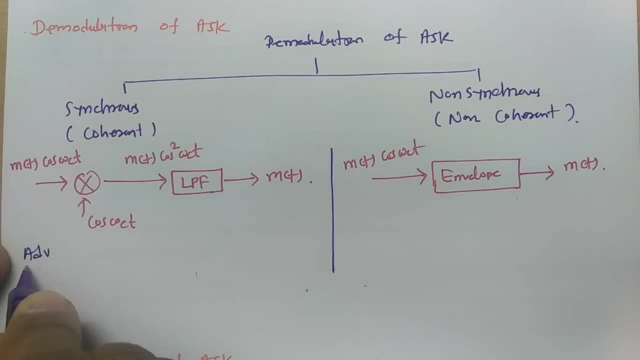 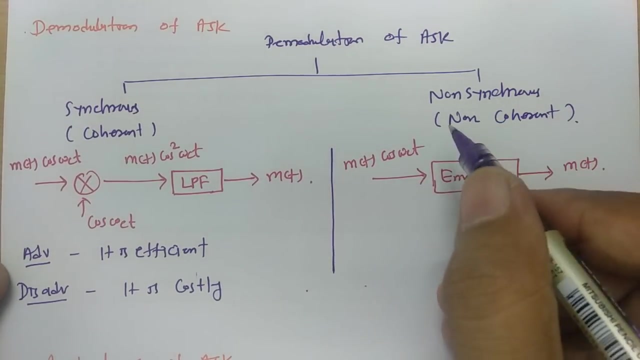 Advantages are: it is efficient, but disadvantage is as follows. that is, it is costly method, while when we talk about non-synchronous method, in that you don't need to have any oscillator, so advantages will be: it is having lower cost, so cost is low. why cost is low? the reason is you don't need oscillator, but disadvantage that is it. 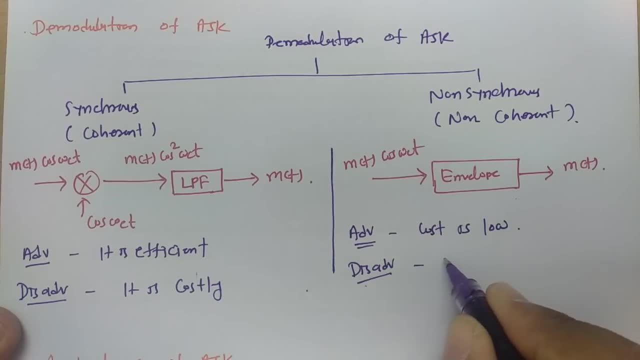 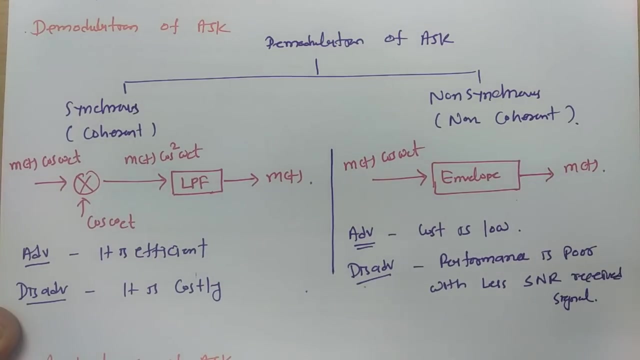 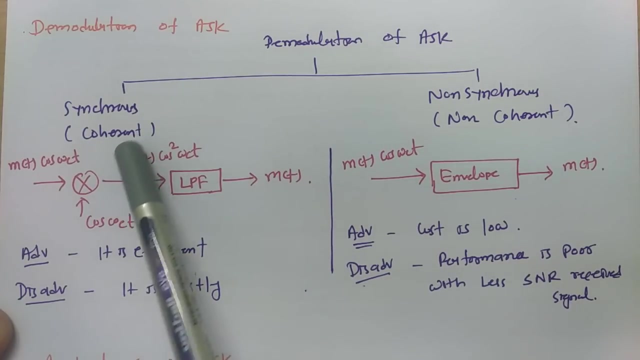 gives poor performance under poor SNR. so performance is poor with less SNR received signal. so this is how advantages and disadvantages are there, with demodulation technique of amplitude shift key. so there are basically two methods: synchronous and non-synchronous. synchronous is having requirement of oscillator to generate carrier signal and that method is efficient. 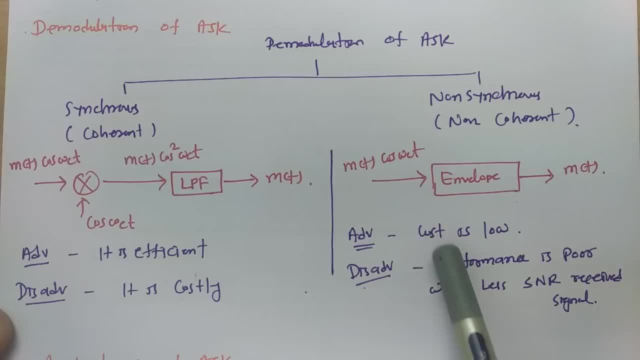 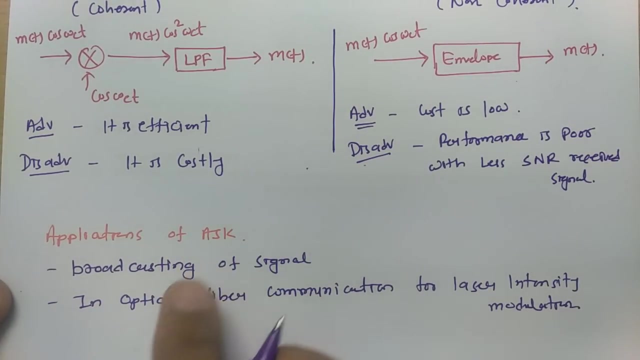 but it is costly, while non-synchronous method that is having lower cost but it has poor performance with less SNR at received signal. Now let us sum up this session with applications. So ASK that has been utilized in broadcasting of signal and in optical fiber communication for laser intensity.